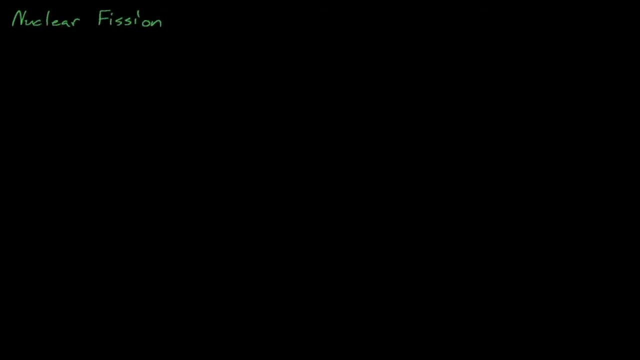 Hello everyone and welcome back to Nuclear Reactor Theory Lectures. So far in this course we've been reviewing some introductory nuclear physics concepts, and today we're going to discuss the physics of nuclear fission, which, as you can probably guess, is a fairly important reaction for fission reactors. 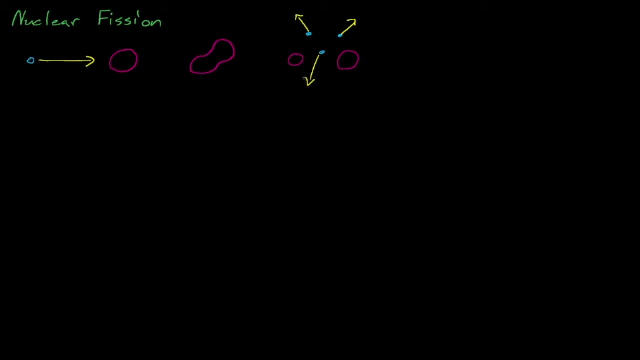 Fission events are initiated when a nucleus absorbs a neutron. The binding energy gained from absorbing this neutron excites the nucleus and provides enough energy to destabilize it. This unstable nucleus assumes this barbell shape as it begins dividing into two halves and eventually these two halves break apart, releasing some interesting radiation as they do. 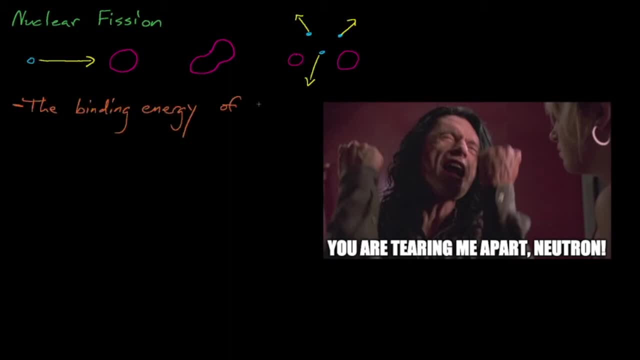 The neutron that induces fission, which is known as the last neutron absorbed by the nucleus before fission, contributes the binding energy that destabilizes this nucleus And thus, if a nucleus is to undergo fission after absorbing a neutron, the binding energy, or Q-value. 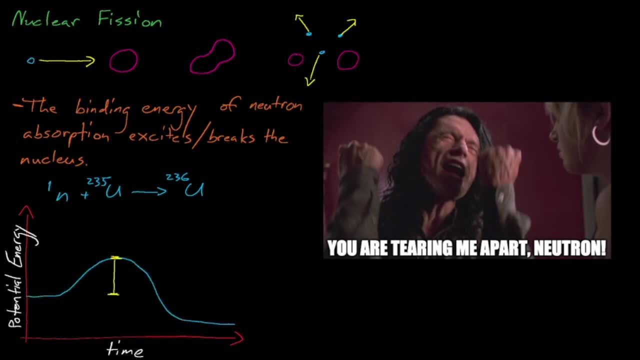 gained by absorbing this neutron must be above some threshold F- This is called excitation energy- which is usually around 6 to 9 MeV. The binding energy gained from absorbing this last neutron isn't always enough to cause fission and, in general, 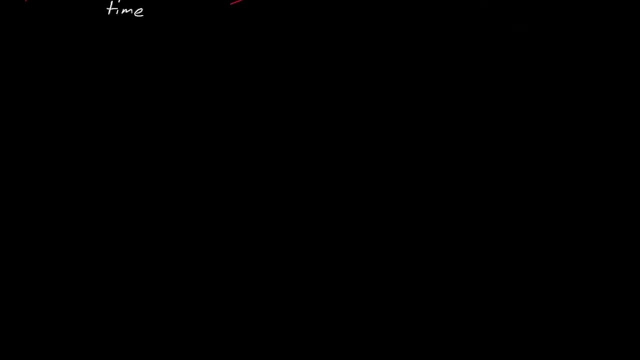 there are two classes of nuclei that can fission. Fissile nuclei can fission from the binding energy alone of absorbing this last neutron, while fissionable nuclei require a little more energy to get over this hump. These fissionable nuclei can, in fact fission if the instant. 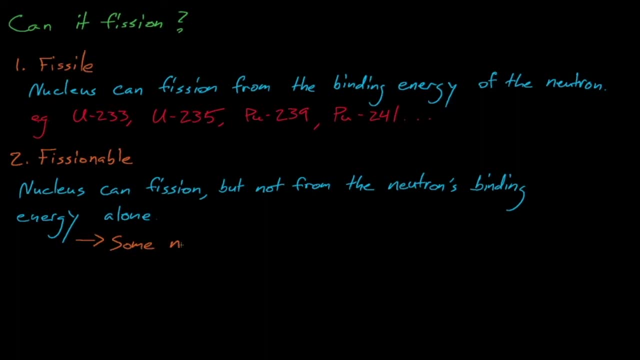 neutron contributes some significant amount of kinetic energy. This kinetic energy is used to excite the nucleus a little more than the binding energy alone excites it. The most common example of a fissionable nucleus is uranium-238, which cannot fission by absorbing a thermal energy neutron, but can fission by absorbing a fast neutron. 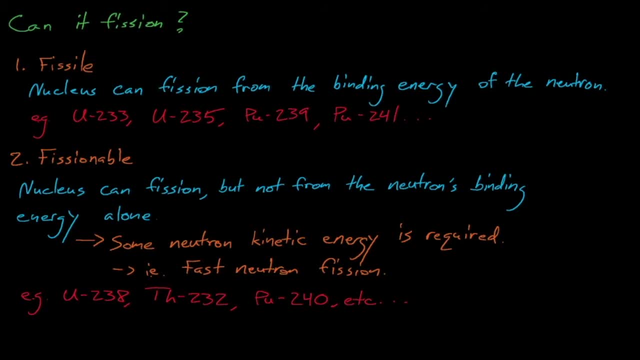 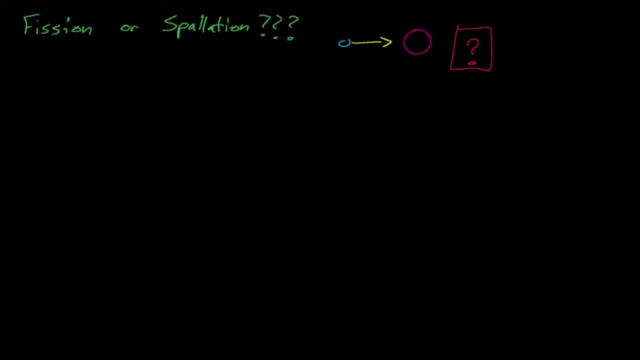 This concept of using fast neutrons to fission fissionable nuclei is used extensively by burner reactors, which seek to reduce the amount of actinides present in spent fuel by fissioning them using fast-spectrum neutrons. Before we move on, it's worth answering the question of how we know if a nuclide fissioned. 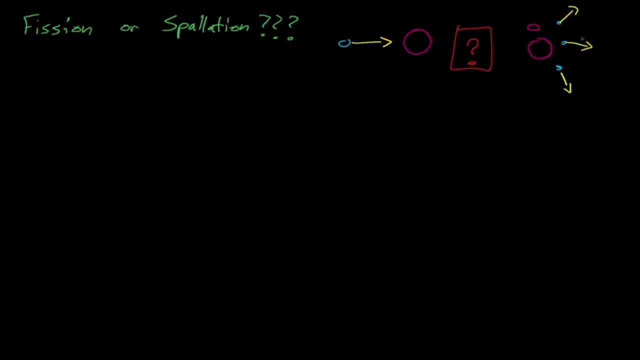 Fission involves forming a compound nucleus which then takes this barbell shape and then eventually splits up. So how can we tell if the neutron was emitted from fission versus if it was knocked out of the initial nucleus? The answer is: time, If the neutron has been emitted by being knocked out or 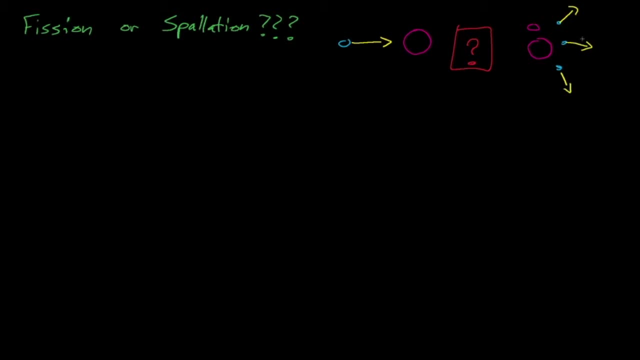 spallated from the target nucleus, then this emission will have no time to form a compound nucleus and is just caused by the kinetic energy from the neutrons slamming into the nucleus. A compound nucleus survives for about 10 to the negative 14 seconds before fissioning. 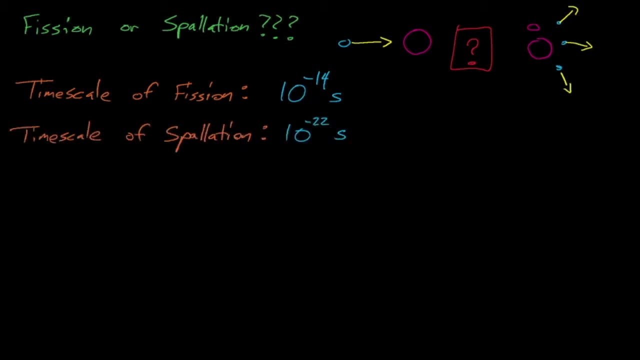 whereas it only takes between 10 to the negative 17 and 10 to the negative 22 seconds for a neutron to traverse the nucleus- a factor of 1 million or more less time. Believe it or not, we can actually observe this significant time difference in a laboratory. 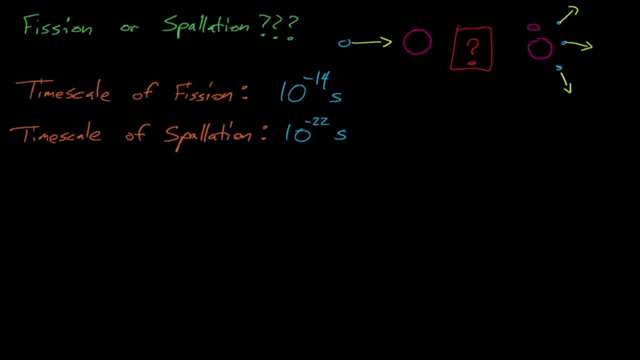 which means that we can actually observe the time difference between a neutron and a fission. We can actually see the time it takes for a compound nucleus to undergo fission. So, to summarize, we have discussed how a nucleus needs to absorb enough energy from a neutron to undergo fission. 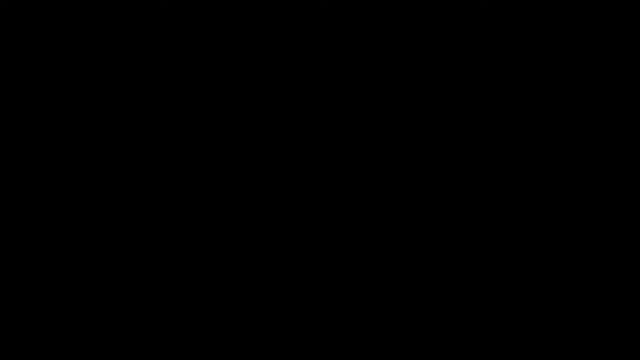 If the energy gained by absorbing this neutron with its kinetic energy isn't at least between 6 to 9 MeV or greater, then the fission cannot occur. However, fission is a particle physics phenomenon and we all know the infamous rules of particle physics. 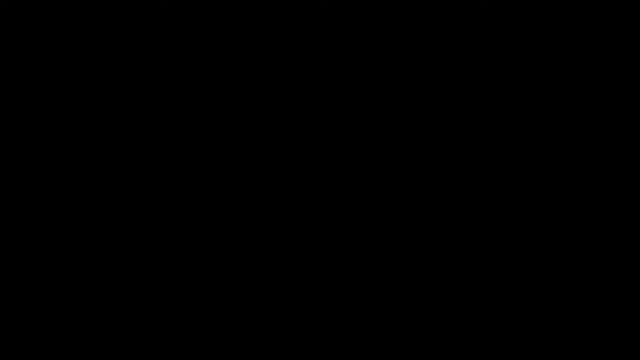 The first rule of particle physics is that you don't talk about particle physics, And the second rule of particle physics is that there are no rules to particle physics. Spontaneous fission reactions are one example of the weird black magic that is particle physics. 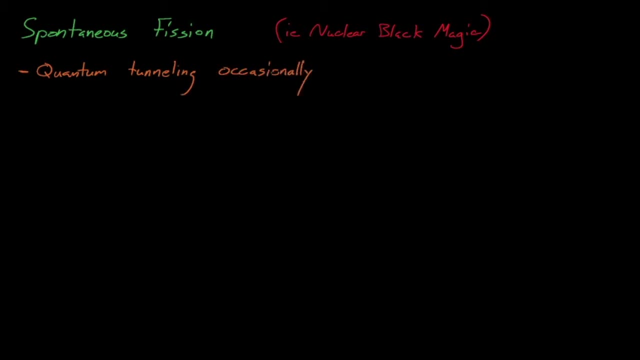 Occasionally, quantum tunneling will allow a nucleus to have enough energy to destabilize and undergo fission, meaning that nuclei can fission spontaneously without having received enough activation energy to do so and actually without having absorbed energy. As with most quantum tunneling phenomenon, the probability of spontaneous fission occurring is very, very low. 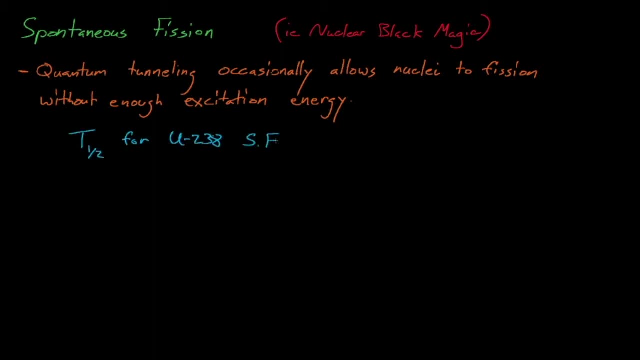 For example, the half-life for a uranium-238 nuclide that undergoes spontaneous fission is about 6.5 times 10 to the 15th years. This seems like a really, really long time. However, most materials have about 10 to the power of 22 atoms per cubic centimeter. 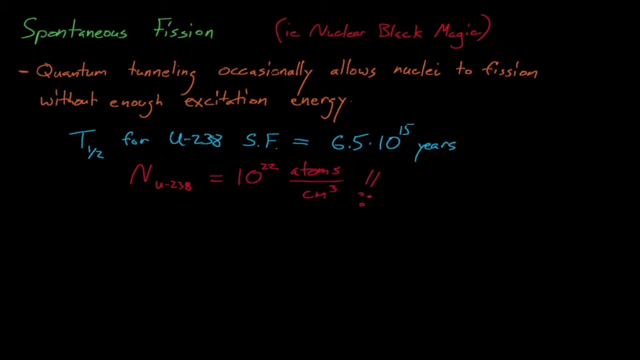 which means that several cubic centimeters of uranium-238 can expect to see a spontaneous fission reaction every few seconds to minutes. Believe it or not, these spontaneous fission reactions have a significant impact on nuclear engineering fields, For example in nuclear nonproliferation. 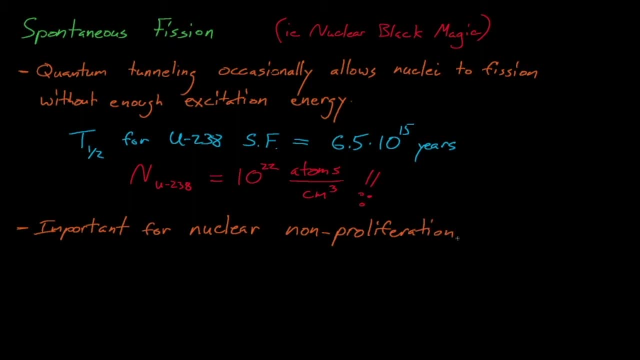 we seek to detect and prevent the proliferation of nuclear material, which might occur by smuggling some amount of uranium across a country's border. The fact that there are always spontaneous fissions occurring in this material and that the spontaneous fissions are likely magnified by inducing a fission in other regions. 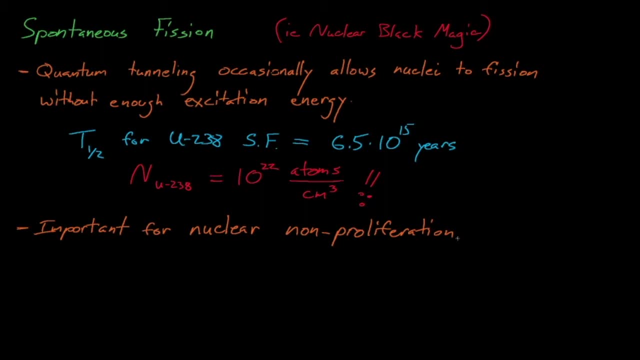 in other fissile nuclei means that this material produces a source of neutrons that can never be turned off, and we can build detectors and portal monitors to try and detect and observe this unending neutron signal. Getting back to our fission physics, 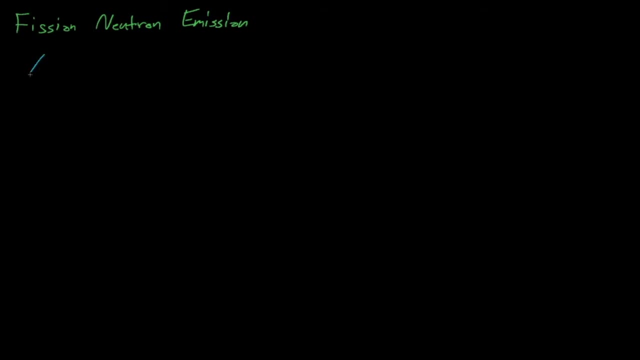 let's discuss the neutrons that are emitted from the fission reaction. The chi distribution or the chi spectrum, describes the energy spectrum of neutrons that are emitted from fission reactions. Chi of E times dE is the probability that a neutron emitted from a fission event will have some energy within dE of energy E. 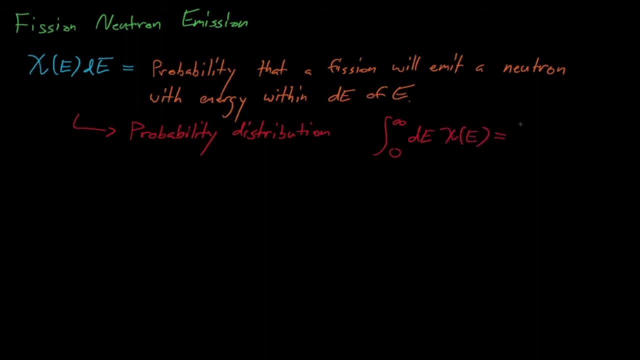 Because chi is a probability distribution and is thus normalized, we see that the integral of chi, of E over all possible neutron emission energies equals 1.. The chi spectrum depends on the target nucleus and on the energy of the neutron that induced the fission. 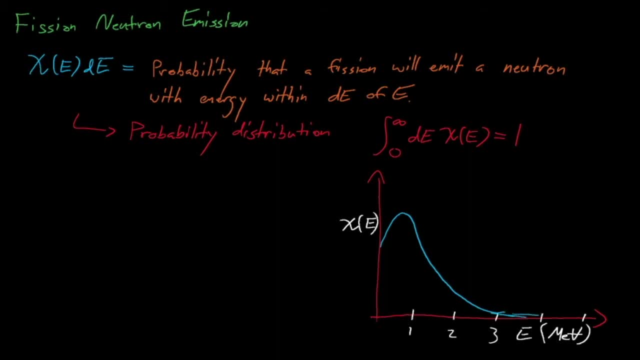 In general, higher energy neutrons tend to cause fission reactions that release higher energy daughter neutrons. In general, the chi fission spectrum follows this shape here, where the mean energy of neutron emission is about 2 MeV and the mode of the distribution occurs around 1 MeV. 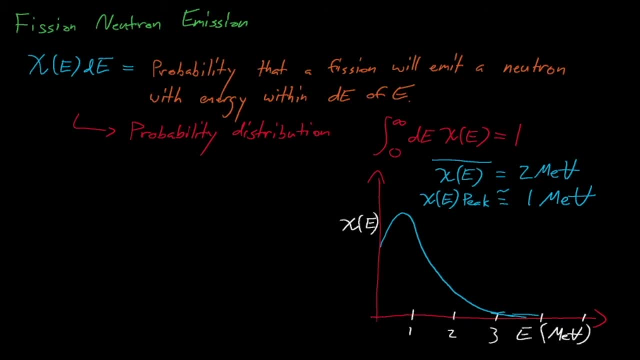 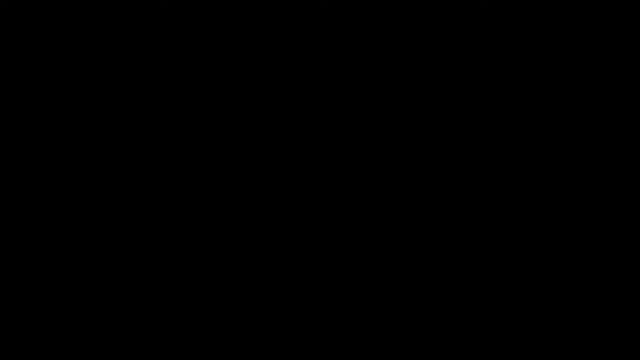 The chi spectrum is effectively equal to 0 at energies below about 100 KeV, which means that essentially all fission neutrons are born at fast energies. Next let's discuss nu bar, which describes how many fission neutrons are released on average per fission event. 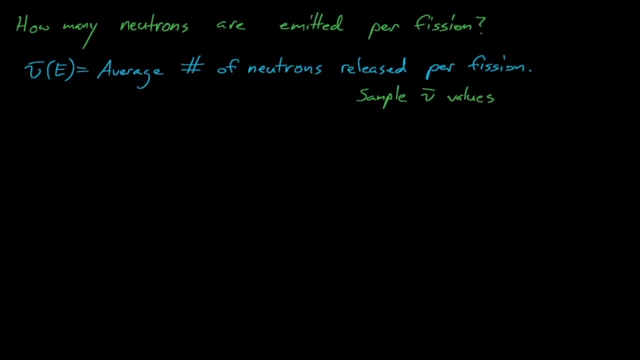 Just like the chi spectrum, nu bar varies significantly as a function of the fissioning isotope and the energy of the neutron that induces fission. However, nu bar tends to vary much more significantly than chi. This table here, taken from Ditterstadt and Hamilton, shows that nu bar varies significantly. 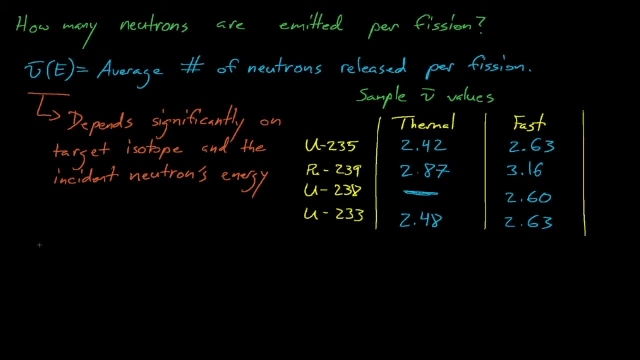 depending on whether a fission event was initiated by a thermal or fast energy neutron, and also that nu varies even more significantly as a function of the fissile species. Note that there is no nu bar for uranium-238, for thermal neutrons, because uranium-238 requires 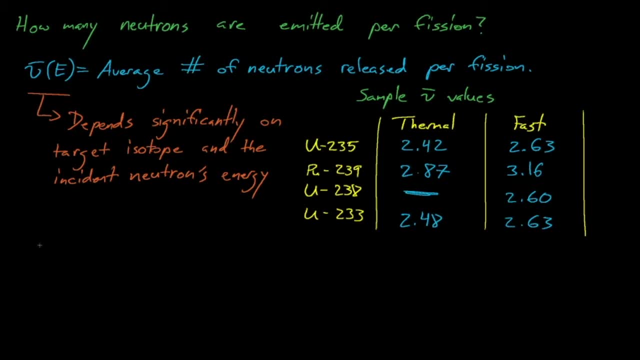 a fast neutron to fission. In other words it is fissionable. We can take this nu bar parameter and tweak it slightly to get the eta parameter, which describes the average number of fission neutrons released per neutron absorbed. The values of nu bar and eta have a significant impact on reactor design. 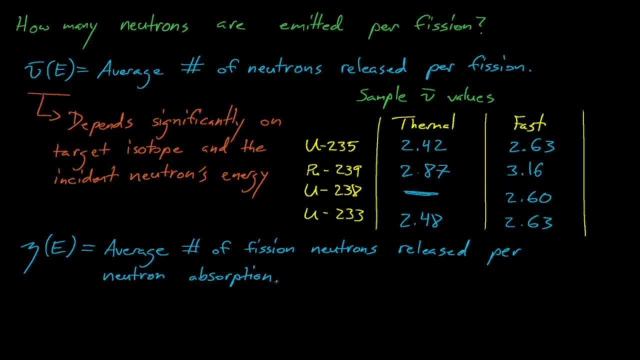 Even relatively small changes in nu and eta can leave us with extra or too few neutrons to feed the fission chain reaction. In fact, having some extra free neutrons in a nuclear reactor provides some very interesting possibilities. We can use those neutrons for neutron diffraction imaging. 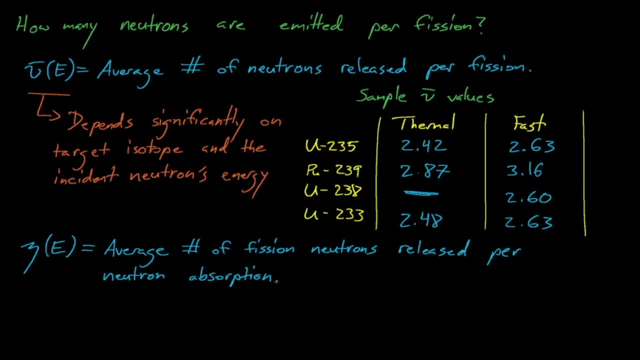 for isotope production for material science studies, and one other interesting possibility is to use those extra neutrons to produce more fissile isotopes. For example, when uranium-238 captures a neutron, it will produce plutonium-239 decaying through a few intermediate isotopes. This means that we can use non-fissile uranium-238. to produce fissile plutonium-239 fuel. In fact, near the end of life for light water reactor fuel, only about 40% of the fission reactions involve uranium-235.. The other 60% of fission reactions are fissioning plutonium-239 that has been bred into this fuel If a reactor's eta value is above. 2, then in theory, we can use one of the neutrons from each fission event to continue the fission chain reaction, and then we can use the other neutron to create a new fissile isotope to replace the nuclide that just fissioned. By doing this we can produce as much or even more fissile fuel. 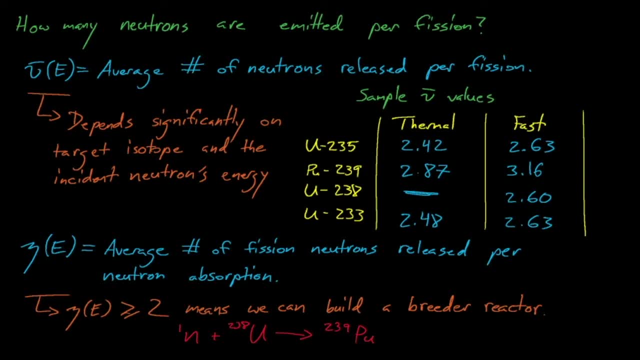 than we consume in this reactor. This kind of reactor concept is known as a breeder reactor. Natural uranium contains about 0.72% uranium-235, and we have enough easily minable uranium-235 to produce a fissile isotope. 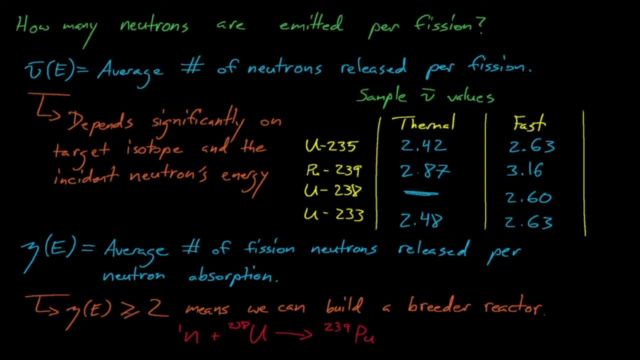 To satisfy the global energy demand for several hundred years. But with breeder reactors we can transmute the uranium-238 that makes up the other 99.3% of natural uranium into fissile fuel. This means that breeder reactors can provide humanity with many thousands of years worth of. energy from fission which can probably last humanity long enough for us to start building Dyson spheres around stars, or until the multivac supercomputer can figure out how to reverse entropy. We will need to build breeder reactors eventually, but for now they are not essential. We aren't going to run out of uranium-235 for a very long time, so now it's generally not worth building or designing more elaborate and possibly more expensive breeder reactors. For now, the once through fuel cycle works just fine. However, when we eventually do want to build breeder reactors, 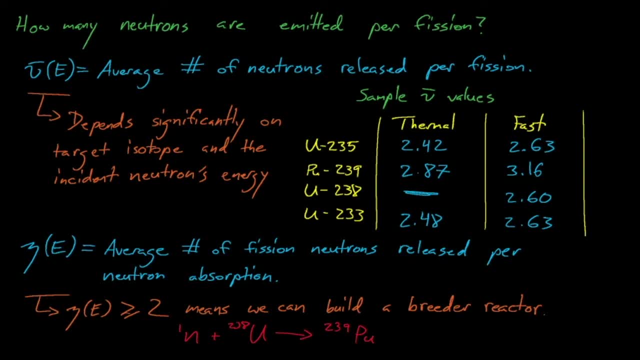 we will probably have to build breeder reactors that rely on fissioning either plutonium-239 or uranium-233.. As you can see in the new bar table, these two isotopes have higher new bar values than uranium-235, and the uranium-235 new bar values are just slightly too small to enable a 235-based. 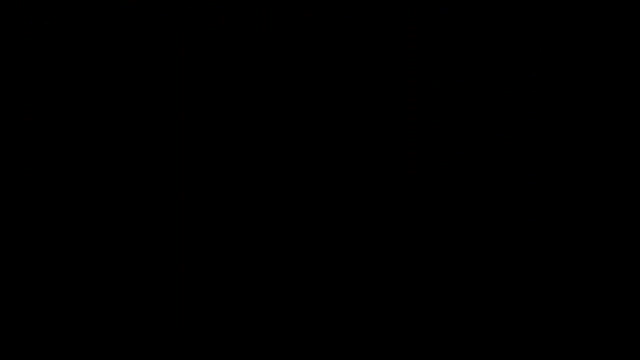 breeder reactor design. The last fission-related metric that I'll discuss today is the capture-to-fission ratio, which is the ratio between the rates of neutron capture and neutron-induced fission in a reactor. The brackets here in the capture-to-fission ratio definition are known as the inner product. 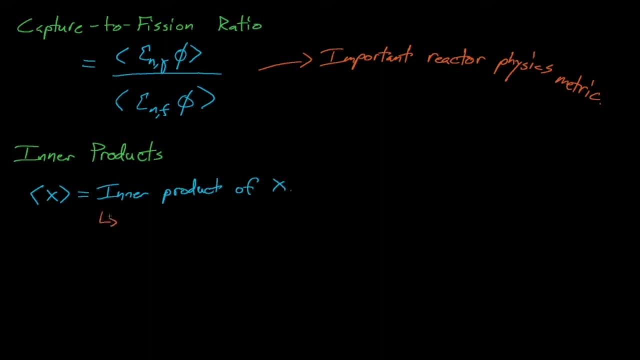 operator. The same notebooks use orbit for fission probability as a much higher parameter for a nuclear reactor. But what is the function for fission? The function for fission basically compresses the energy flow that willゆ скаж y, y and z. 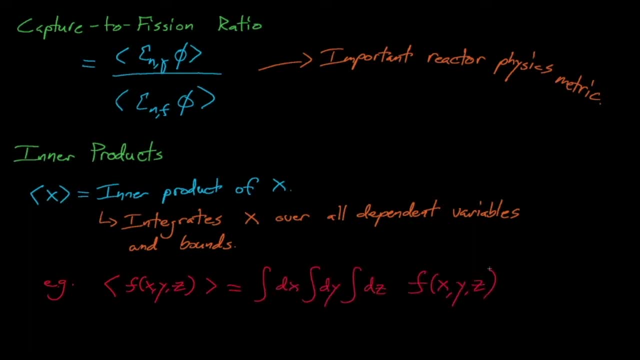 rica QP", for instance, Windows emerg After u sia Well對不起 Basics. So the Muchas Explained Design Theory Frozen Continuous i reactor. The capture to fission ratio is important in reactor design because it describes how effectively nuclei absorb neutrons. A lower capture to fission ratio means that neutrons 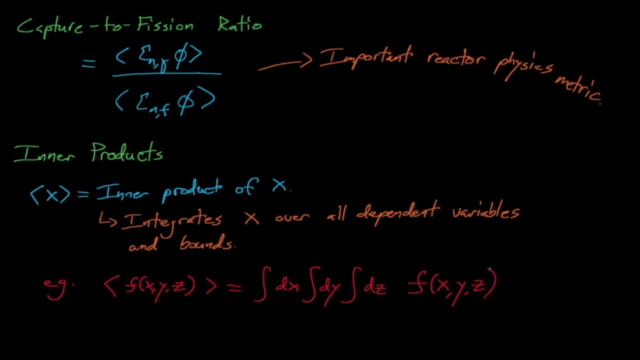 are more likely to cause fission events versus capture events and thus are more likely to continue the fission chain reaction. However, a low capture to fission ratio isn't always necessarily a good thing, and in isotope production, our goal is usually to make sure that nuclei 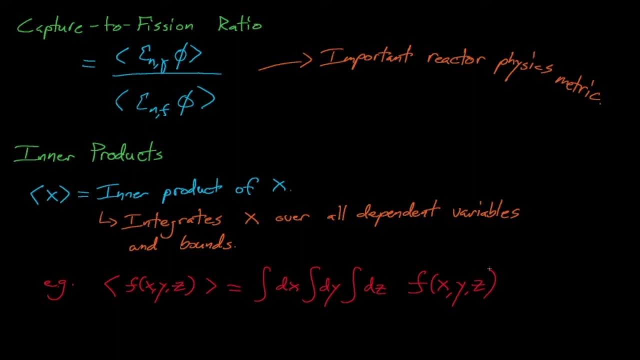 absorb neutrons and that they don't fission so that they can transmute into other isotopes. In this case, our goal is to have a high capture to fission ratio. Our reactor's capture to fission ratio is approximately equal to the ratio of its microscopic cross-sections. However, this assumes 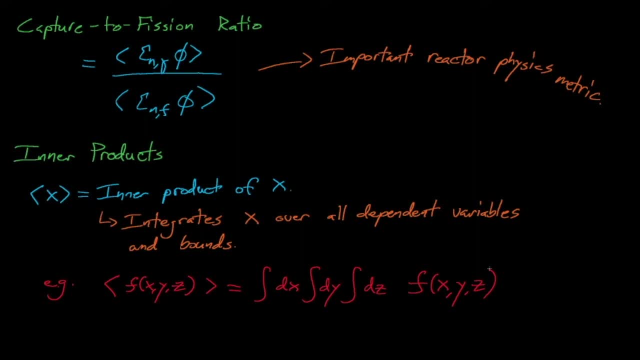 that our reactor contains only one isotope and that our flux has no spatial dependence whatsoever. This is, of course, almost never true, but in general, considering the capture to fission ratio, as the isotope's microscopic cross-sections, allows us to estimate the worth of fissile isotopes and to estimate how a reactor's capture. 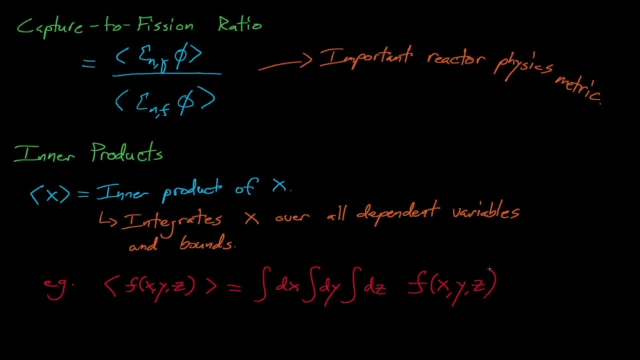 to fission ratio would change in response to different changes in its neutron spectrum. So, now that we've discussed these different fission reaction mechanics, what happens after a nucleus undergoes fission, and what are we left with after a nucleus undergoes fission? 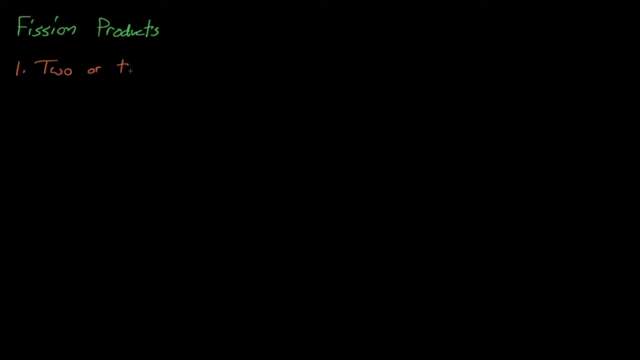 Well, first the nucleus splits into two, but sometimes three or more smaller nuclei, which are known as the fission products. There are an enormous number of combinations that are possible to do with fission. For example, if we were to do a fission reaction, 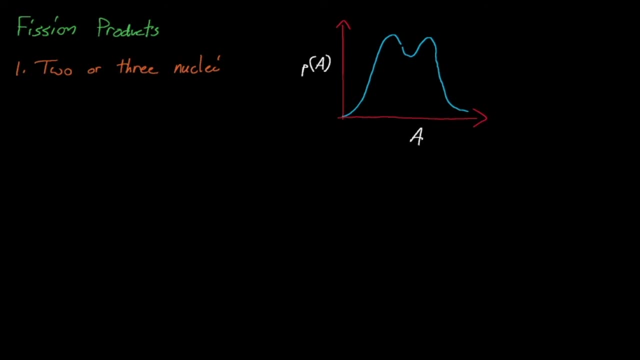 that describes how a nucleus's protons and neutrons can separate into two smaller pieces and thus the possible atomic masses of fission products, follows this double-humped probability distribution, where molybdenum-99 is one of the most common fission products. This 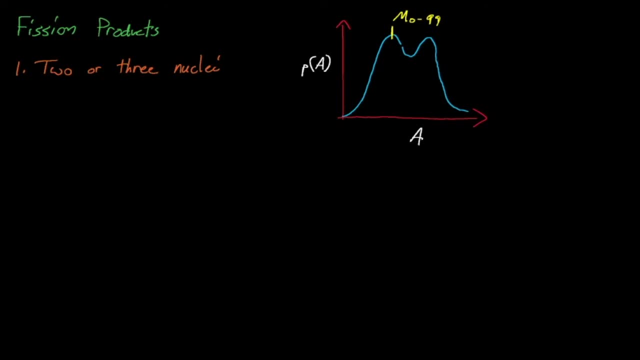 distribution is double-humped because a lower mass in one fission product correlates to a higher mass in the second fission product. It's not shown here, but as we increase the energy of the neutron that induces fission we can see that the fission products are more. 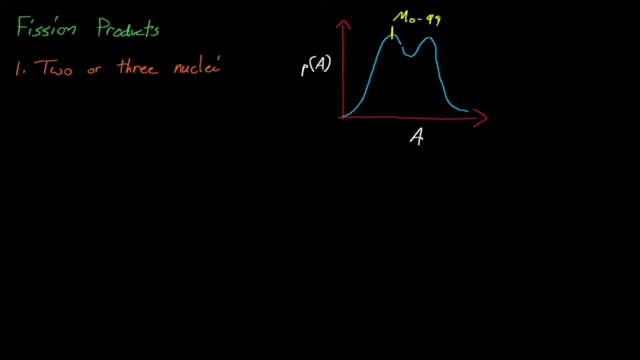 fission-inducing than the neutrons. The trough between these two peaks in this distribution becomes less and less deep. As with all of our fission metrics, this distribution of fission products also depends on the fissile species, which means that different nuclei will produce. 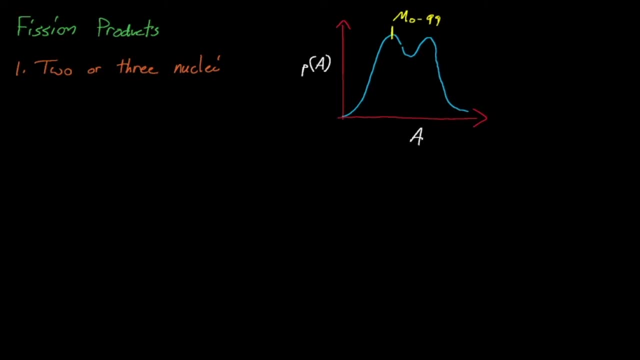 slightly different sets of fission products. In general, nuclei require slightly more neutrons than protons to remain stable, which means that when heavy uranium nuclei fission, that their fission products are going to be very, very neutron-rich, In fact, more neutron-rich than 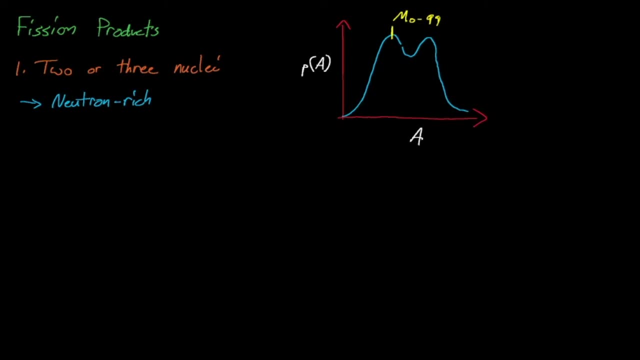 the neutrons are going to be. This means that they will be much more stable than they want to be. So, to approach stability, these fission products will undergo several rounds of radioactive decay, which is generally alpha or beta minus decay, until they reach a stable Z-to-A ratio. This gradual series of radioactive decays is responsible for the overwhelming majority of radioactivity in spent nuclear fuel, and most techniques aimed at reducing the reactivity of spent nuclear fuel will try to either separate out or transmute away the longest living and the most significant heat generating of these radioactive fission products. 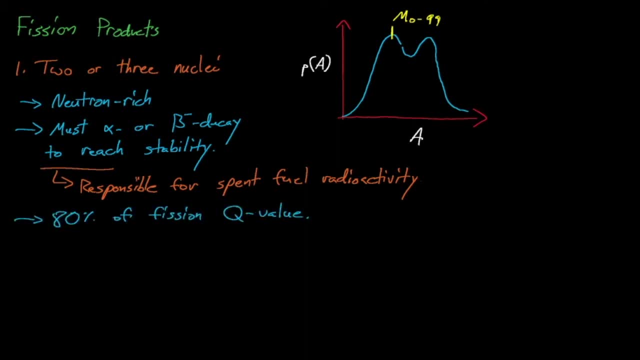 The majority of the energy released by the fission reaction, about 80%, is carried away by the kinetic energy of these fission products. These high energy fission products have an incredibly short range in materials, which means that most of the energy released from the fission reaction is deposited very close. 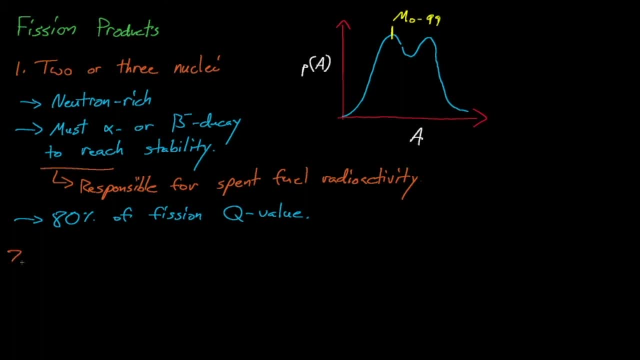 to where the reaction occurs. In contrast, gamma rays and neutrinos that are also released from fission carry about 10% of the energy from fission, and these particles have a much larger range. This longer range means that the particles deposit their energy in different places. 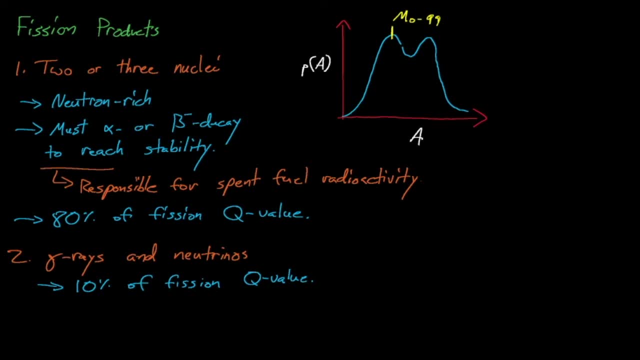 sometimes between centimeters and even meters from where the fission occurred. Neutrinos, which are one of the most interesting particles in all of physics, can carry this energy even further. Neutrinos travel at the speed of light but, enigmatically, also have a non-zero rest mass. 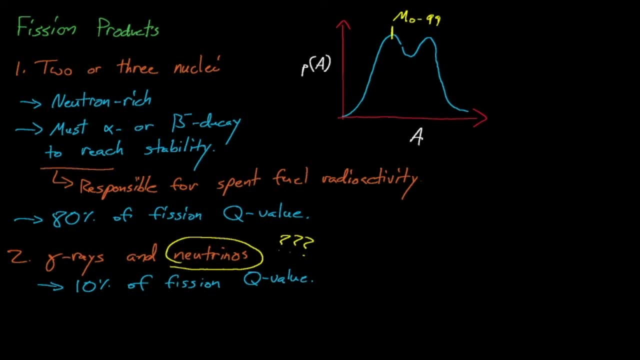 and can keep track of time. Most importantly for us, neutrinos have a very high energy efficiency. Neutrinos have a cross-section that is only very, very slightly above zero, which means that almost every neutrino made in a nuclear reactor will stream directly out of the reactor's.